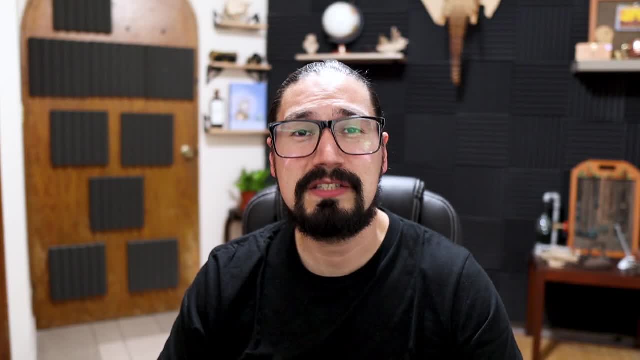 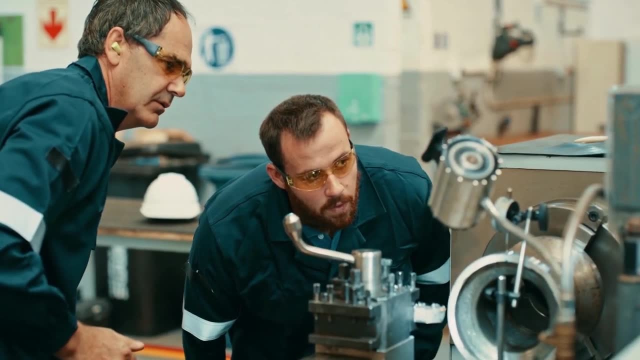 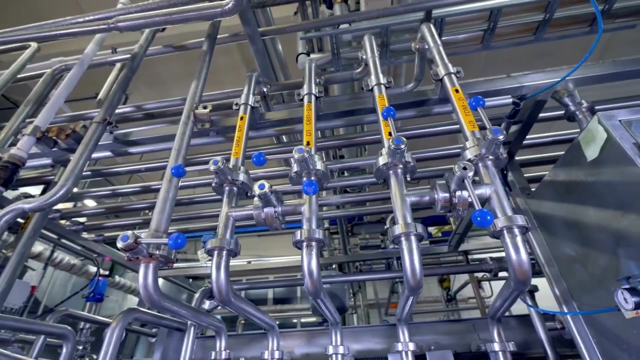 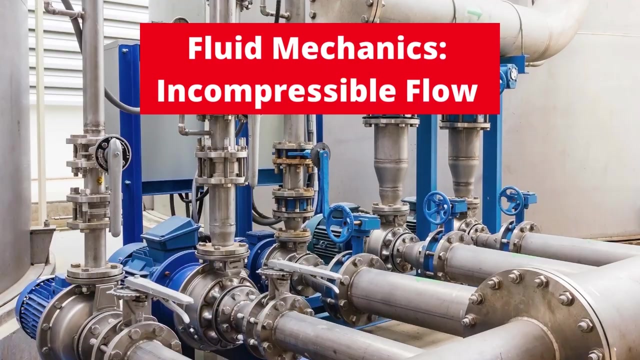 fittings, valves and more. Fluid mechanics is undoubtedly the pillar of such applications. hence the importance of understanding this topic for your engineering career. Welcome to the course: fluid mechanics for incompressible flow. My name is Emmanuel Ortega and I will be your instructor throughout this program. Now, the intent of the course is to explain fluid mechanics for incompressible flow. The intent of this course is to explain fluid mechanics for incompressible flow. Now, the intent of the course is to explain fluid mechanics for incompressible flow. 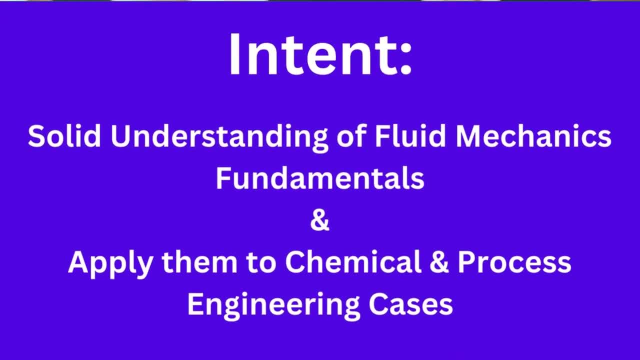 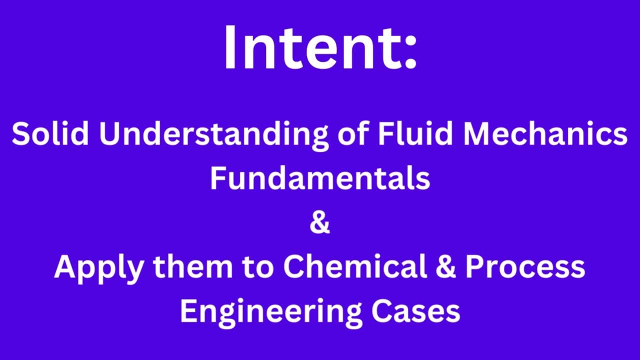 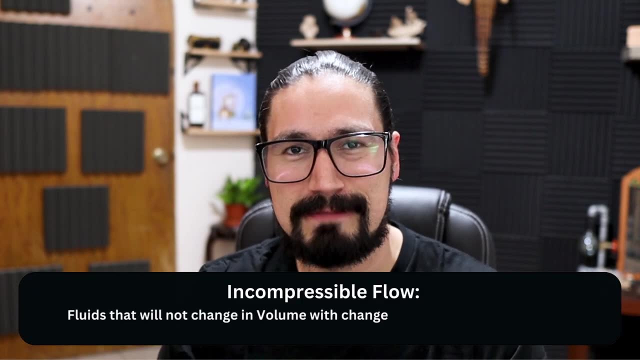 this course is clear: to have the solid fundamentals and understanding of the engineering that goes behind fluid mechanics, but focus towards process and chemical engineers. this very first part is going to be focusing mostly towards incompressible flow, which is essentially liquids, and although this may sound a very niche application, it's one of the most important aspects to consider. 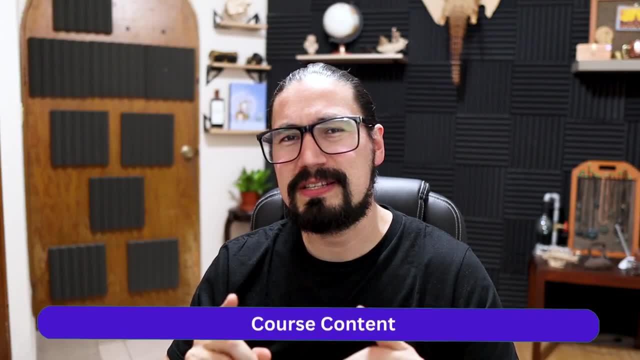 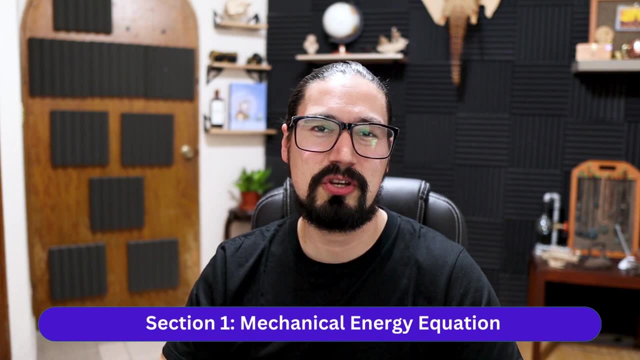 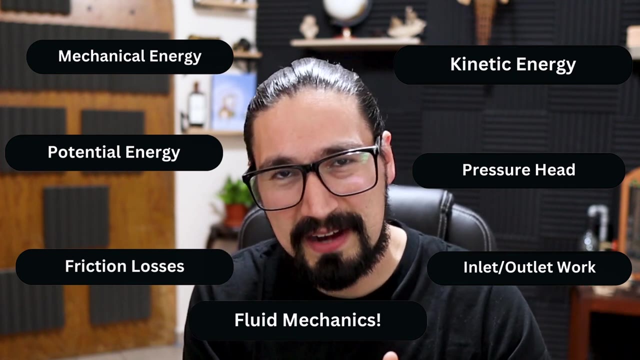 whenever working with this type of products. now let's get a little bit more technical and dig deeper into the topics that we're going to be covering. number one will be the general introduction to the mechanical energy equation: understanding mechanical energy concepts, the importance of kinetic energy potential, energy pressure, friction loss and inlet and outlet work. 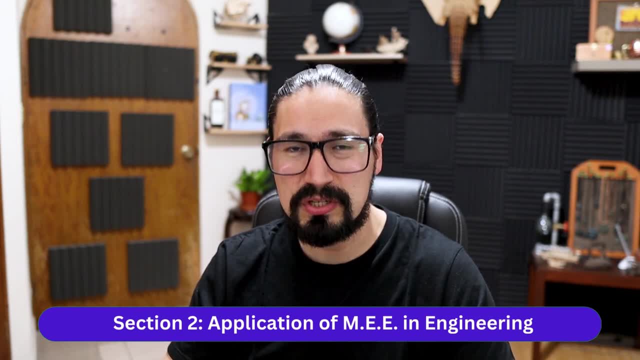 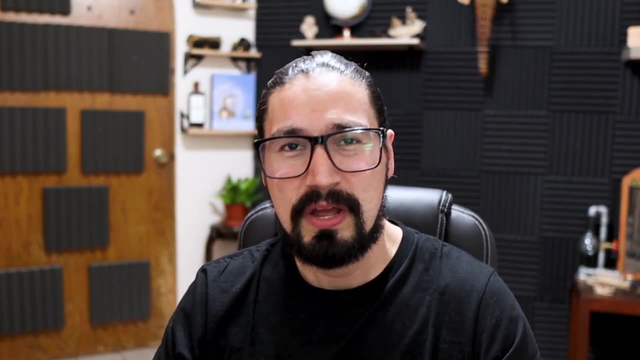 after understanding the fundamentals of the mechanical energy equation, we're going to get started with the application of such equation, since this is a very practical course. we're going to be focusing our attention on the mechanical energy equation and we're going to focus our attention into very common engineering applications. we're talking about moving a fluid. 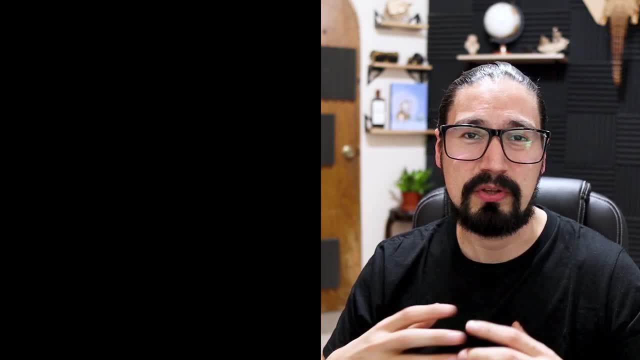 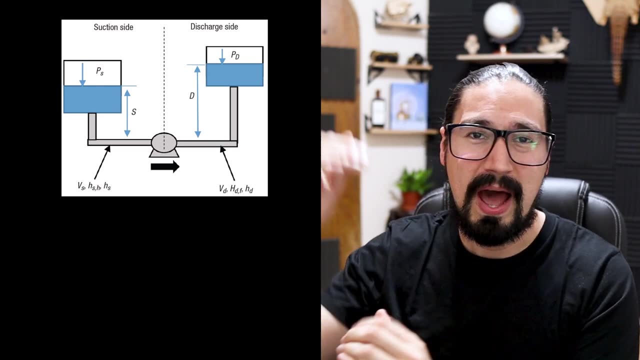 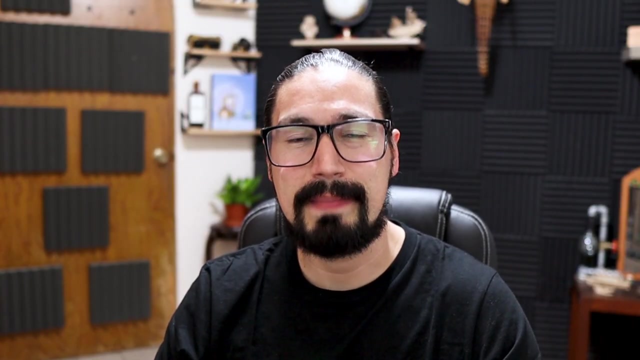 from point a to point b via pipeline. we're talking about maybe emptying a storage tank. maybe we're talking about sizing a pump, understanding how much height could we work with such pumping systems, and much more. the main idea of this section is to work with the mechanical. 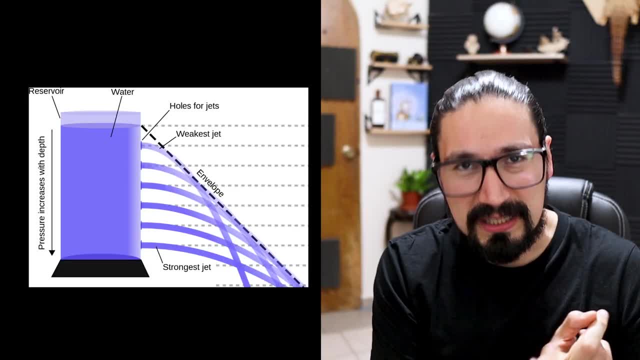 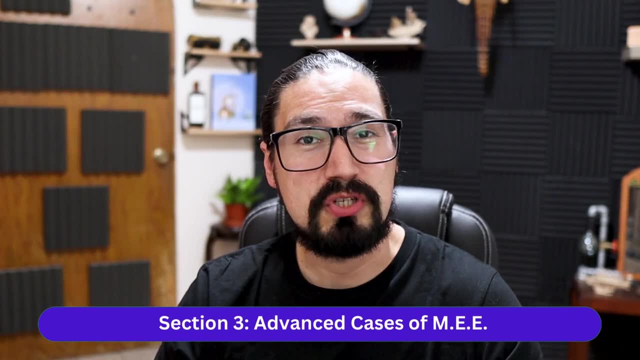 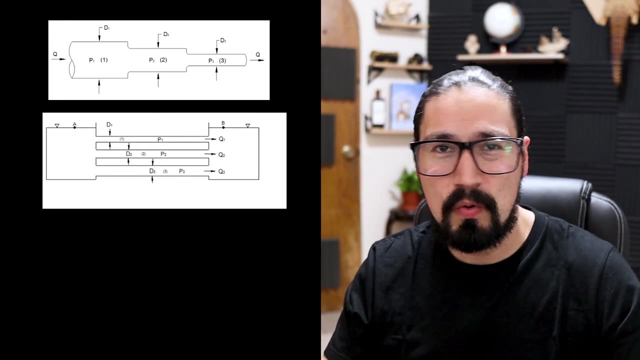 energy equation in simplified versions, for instance Torricelli's law, Bernoulli's law and, of course, the application of the equation. and finally we go to section number three, which covers more advanced applications of the mechanical energy equation. we're talking about serious flow, parallel flow.